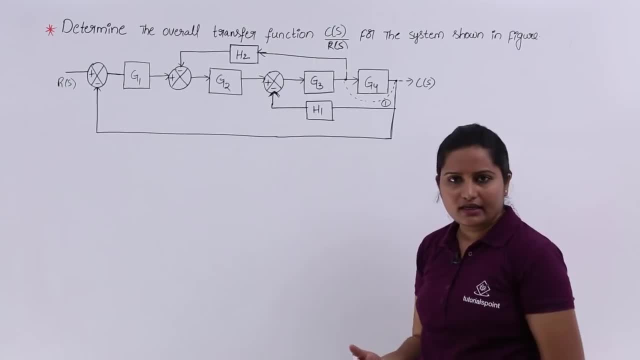 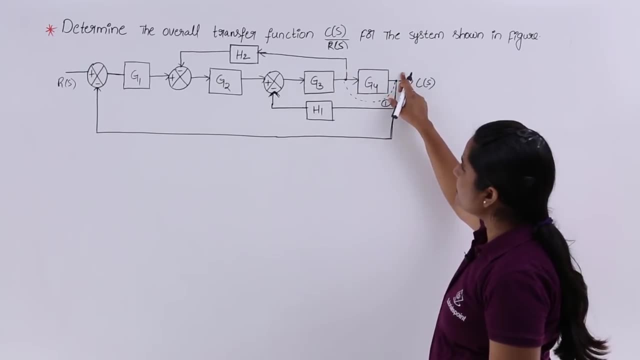 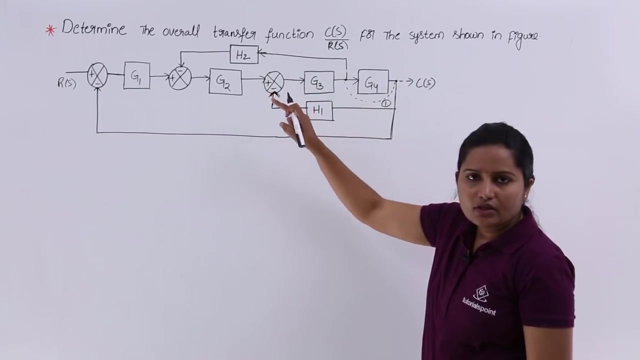 reduction rules. we can apply any of the rule, any. at any place. we can apply any rule. So, for example, you can see, you can move this point to here to release these blocks, or you can move this point to here to reduce this feedback loop. So which you want, you can do. So I want to move my 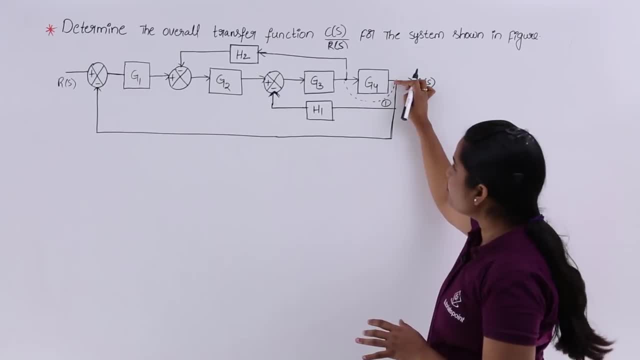 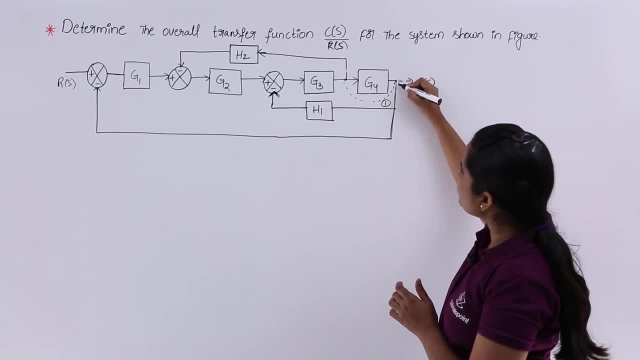 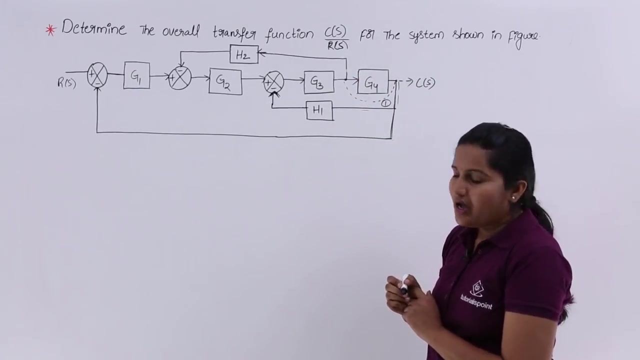 means you just treat. these are two points, So one is for feedback, another one is for H 1. So I am just making this line as it is, but whatever connection to this is there that I want to move here? I do not want to move this feedback, I just 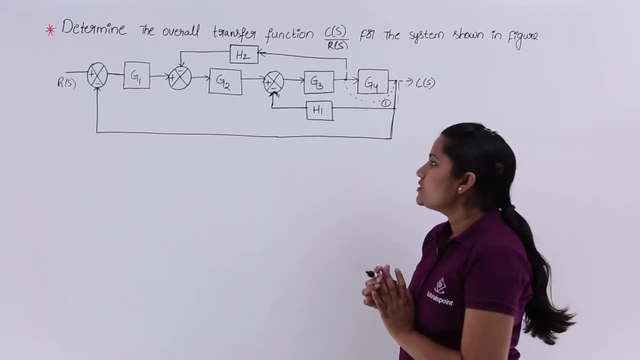 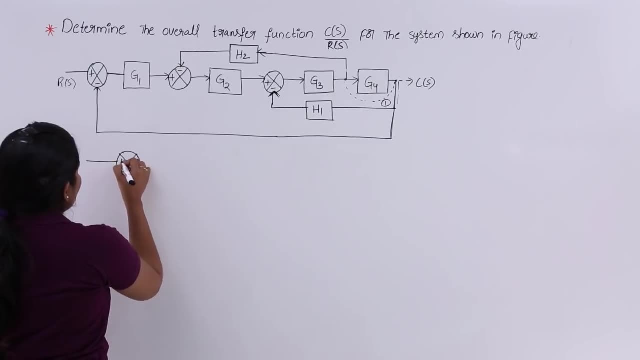 want to move this line to here to here. So I am just making this line as it is, but whatever connection to this is there that I want to move this point to here. that is it. So now you can see how my block diagram is going to change. So now I am having a summing point here, and here I am. 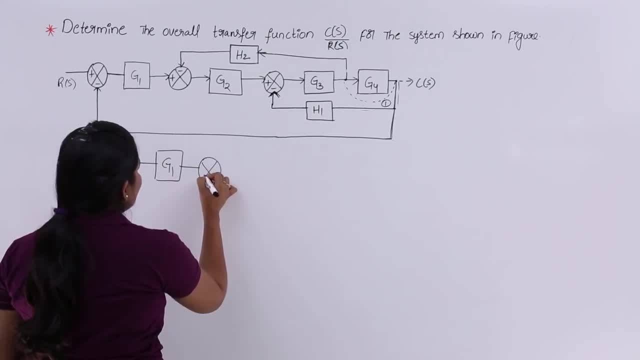 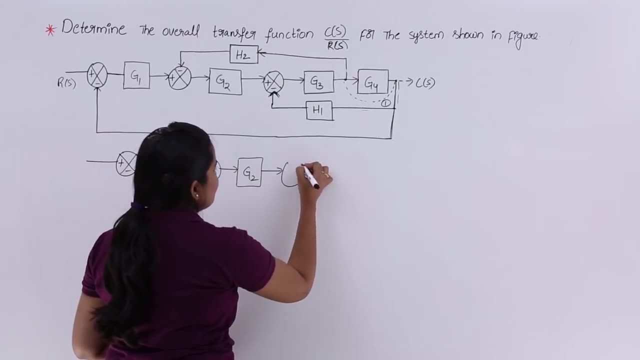 having gain G 1, and here I am having another summing point, and here I am having my gain G 2, and here I am having another summing point. So here, gain G 3, and here I am having my gain, G 2.. 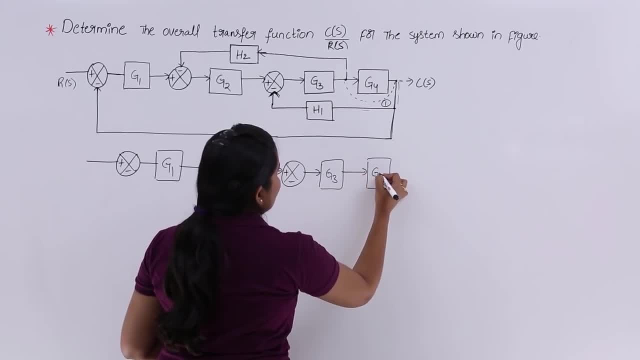 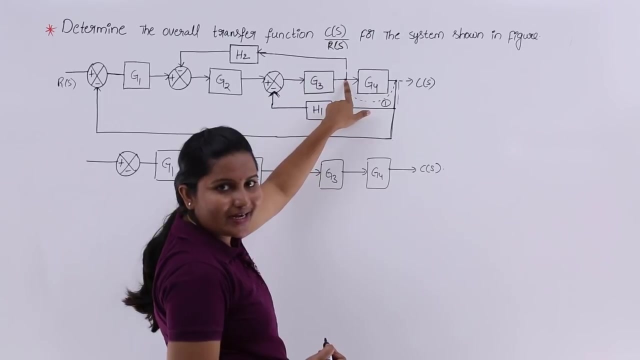 Here my gain: G 4.. So here C of S is there. Now you can see, if you want to move this point to here, what we need to do. So we need to add an extra block with multiplication of G 4.. So here I am. 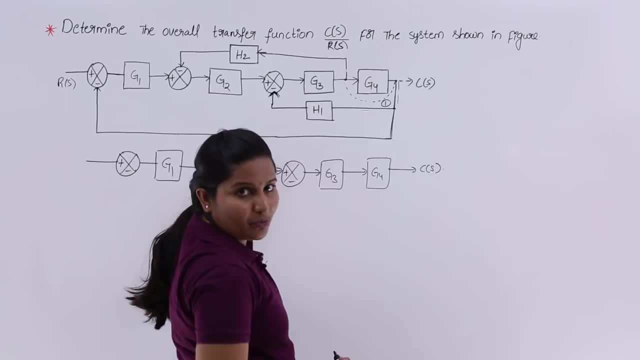 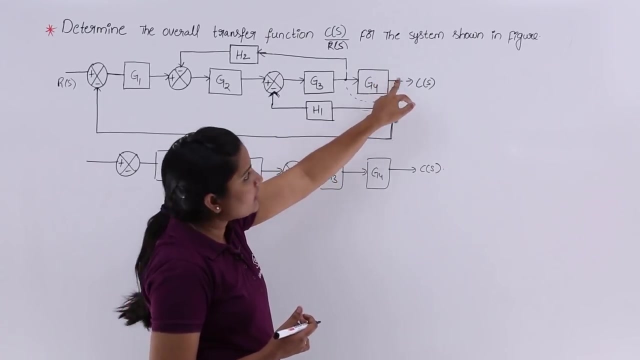 not having anything. So here I need to make a block that is as G 4.. And here H 1, G 4.. So you just observe that rules when you are moving before the block. this point is having effect of this G 4, but you are moving this point to the area which. 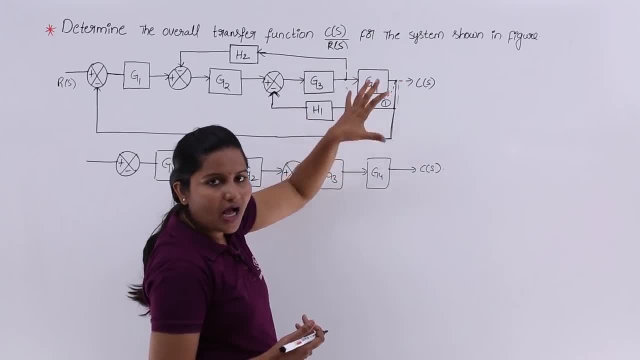 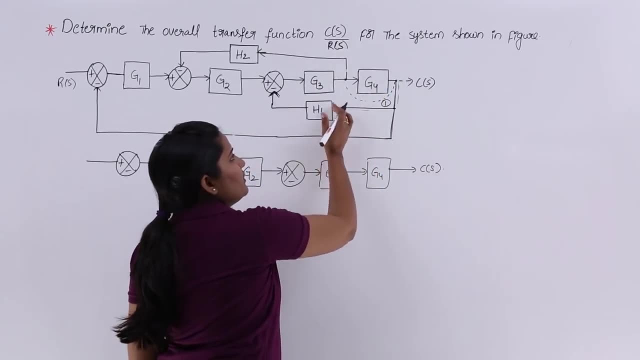 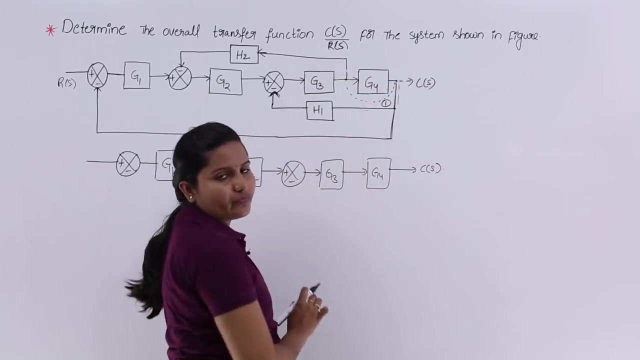 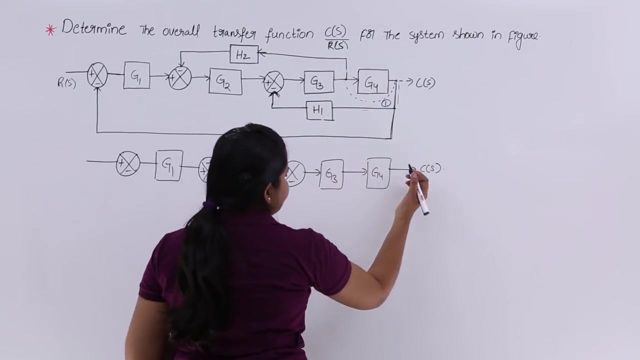 is not having effect of this G 4.. So how we can show the effect of G 4?? So that means by adding here itself will show the effect of that G 4.. So when you are moving this point to here, you need this effect also. So that is H 1 into G 1.. So now, here you can. 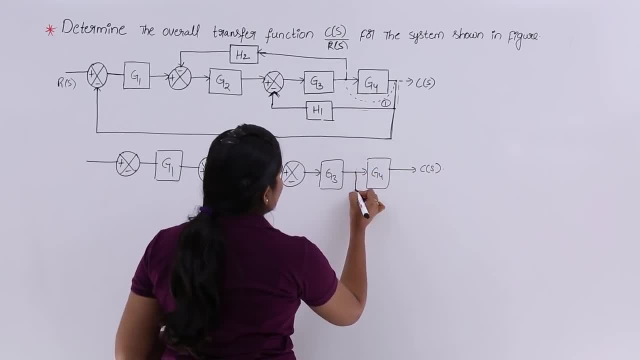 see I am moving this point to here. So this point to here means so here I am having this H 1.. So H 1, H 1 into G 4.. H 1 into G 4 and here, whatever the feedback is there, total overall feedback is there for. 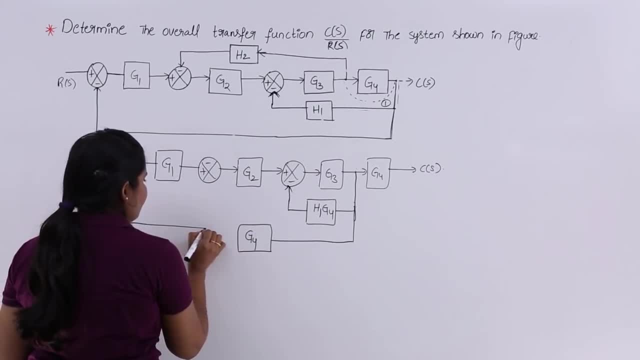 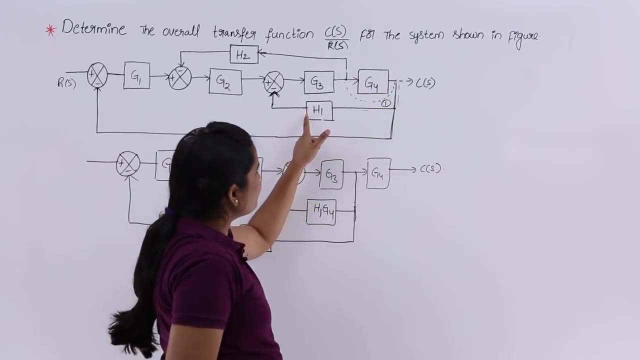 that also I am multiplying G 4.. I move this point to here thus, that is why I given effect of this G 4 to both lines connected to this point. So for this H 1 into G 4, for this here I am not having any block. that means you just treat that line gain as 1, 1 into 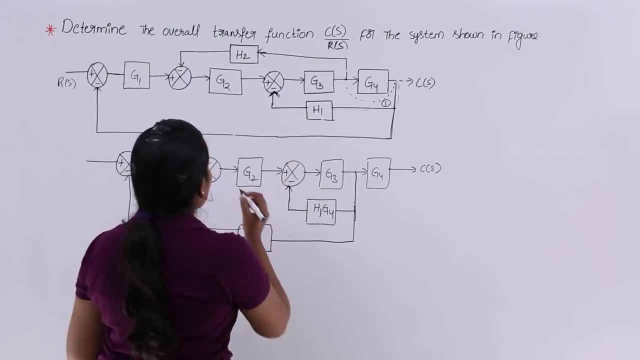 G 4, G 4.. So, like this, I modified the diagram and here I am having a feedback, I think. So here I am having H 2.. So this H 2 is from here. So now you can see. 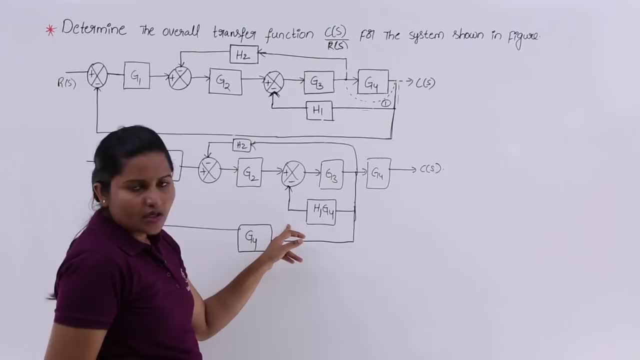 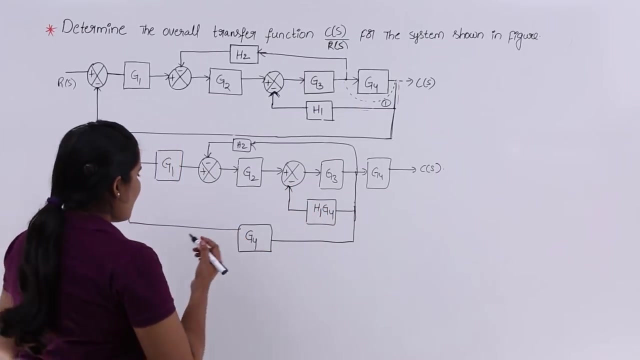 Your feedback path is free now. So this feedback path you can reduce to negative feedback gain. So that means G 3 divided by 1 plus G 3, H 1, G 4.. So I am reducing this block diagram like this. So here I am having a summing point and here I am having G 1 and 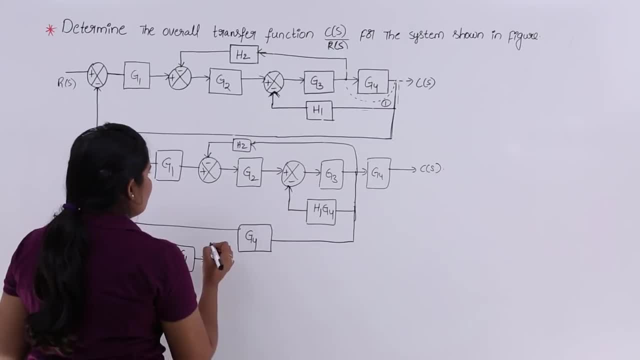 here I am having a feedback. So here I am having a feedback, and that feedback is H 2.. I am taking this G 4 little bit up for my convenience, So here now I can write my block diagram. So this is H. 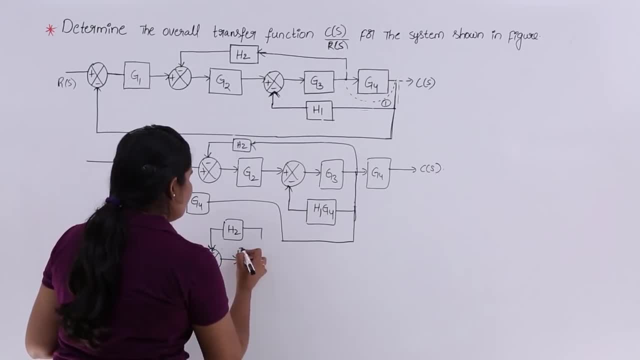 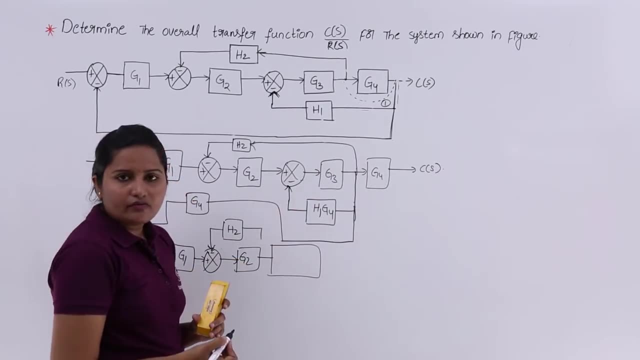 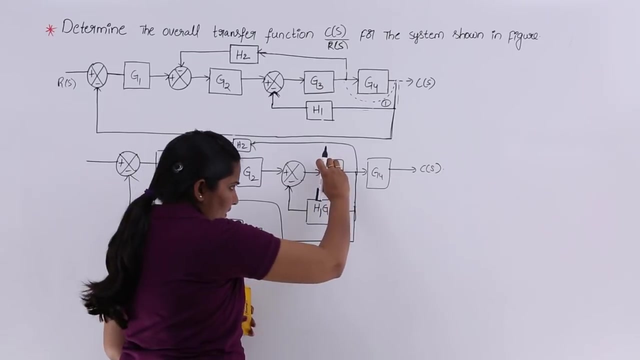 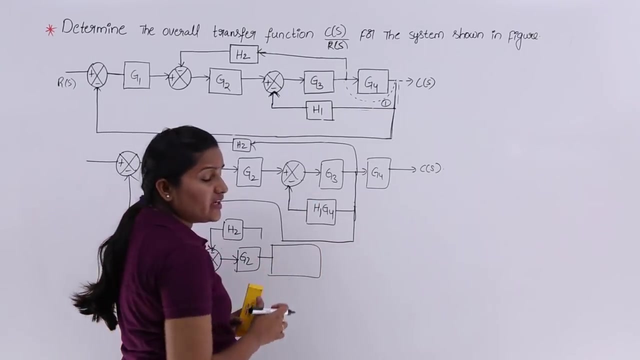 2. So this is G 2, and here I am modifying my feedback. So this feedback, we can reduce this with feedback gain. Feedback gain is this is negative feedback. If you treat this is G and this is H, G by 1 plus G, H will be the feedback gain, But here, in place of H, 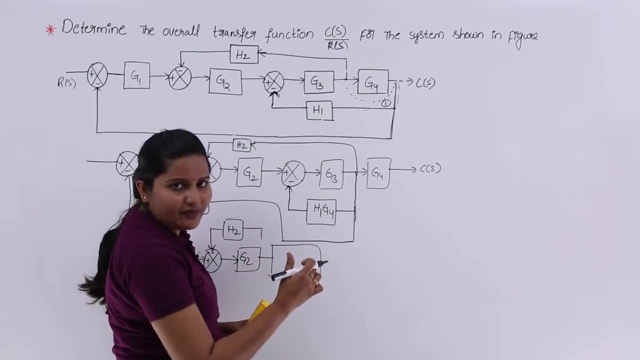 you are having H 1- G 4 that you need to consider as feedback path gain. So now here the feedback path gain is G 1- G 4.. So this is G 2, and here I am modifying my feedback. So this is: 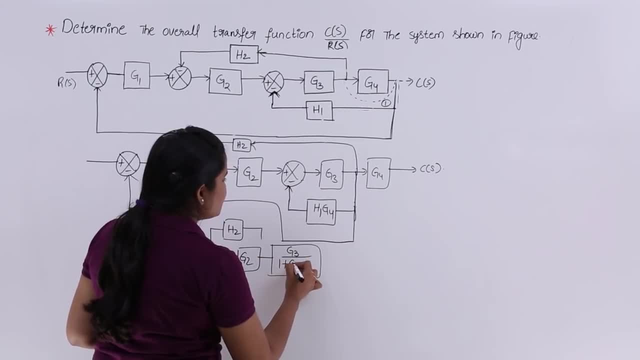 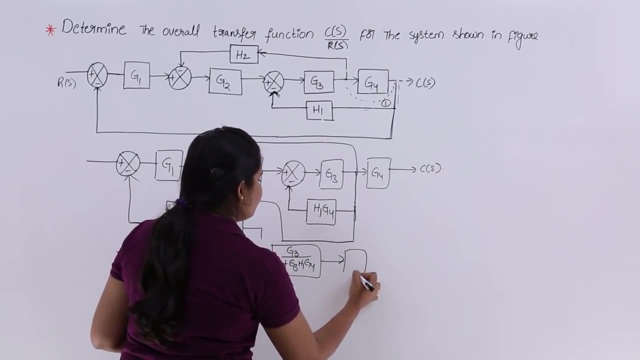 he is giving my feedback. path gain is G 3 by 1 plus G 3 into H 1, G 4.. So now we are having G 4, Now we you are having G 4 and C of S. So this line is at here, So you. 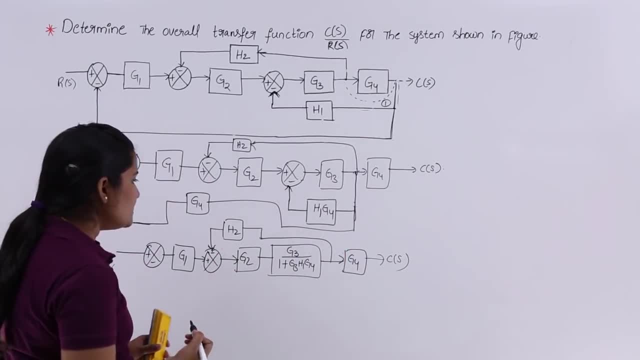 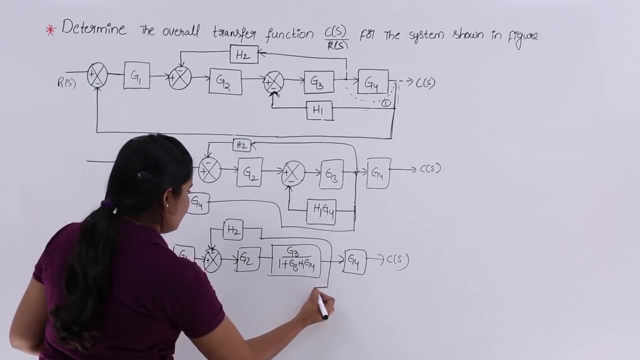 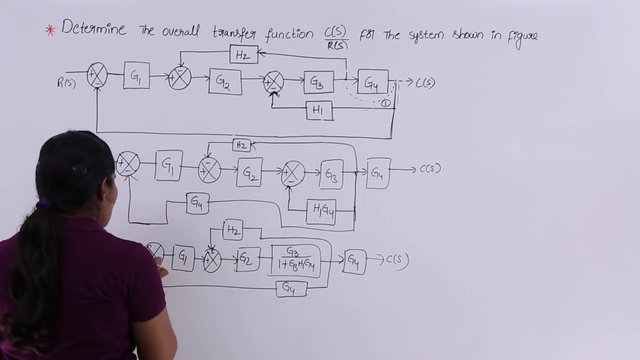 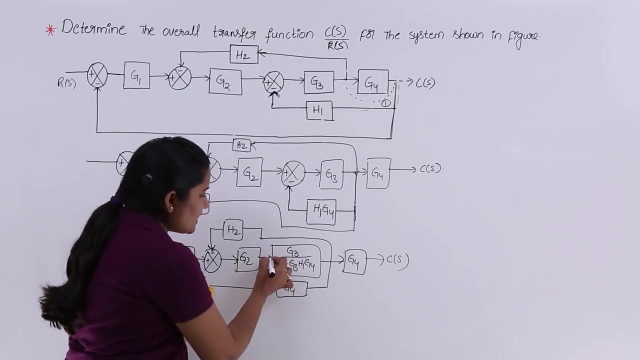 are having like this, And here you can see: is there any other line we missed means So. So this is G 4 and here also we are having G 4.. So G 4 we are having like this: This is RFS diagram, reduced diagram. Now you can see. you can see these two blocks are in series. 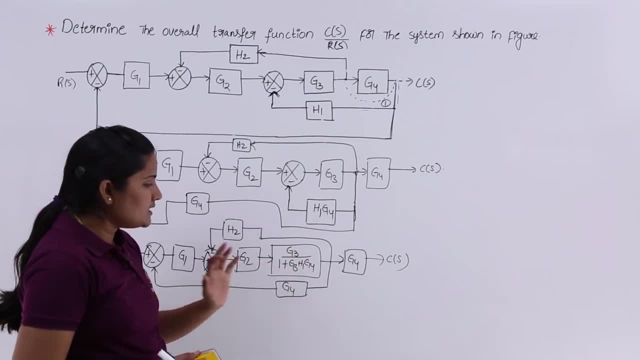 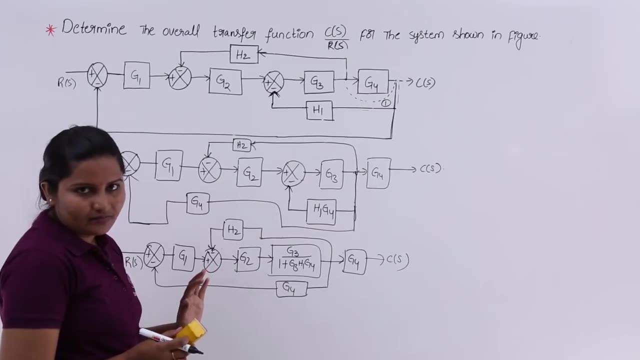 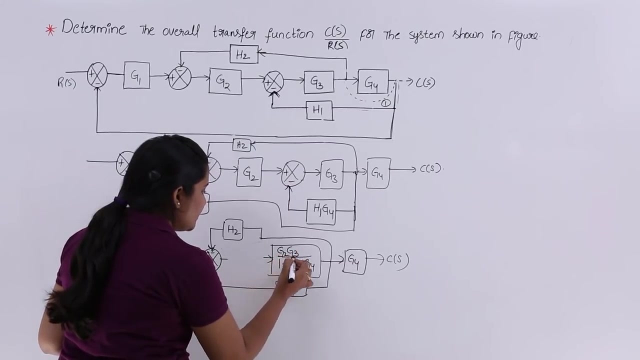 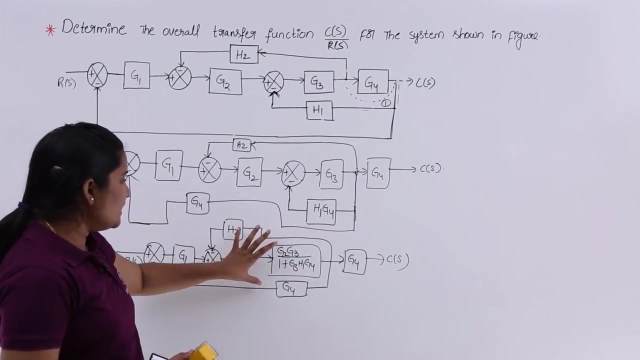 When you are having two blocks are in series, you can make them as a single block by multiplying those two blocks gain. So in the next step I am taking out this block, I am adding that G 2 here, G 2 into G 3, divided by 1 plus G 3, H 1, G 4.. So now, here you can see, here you. 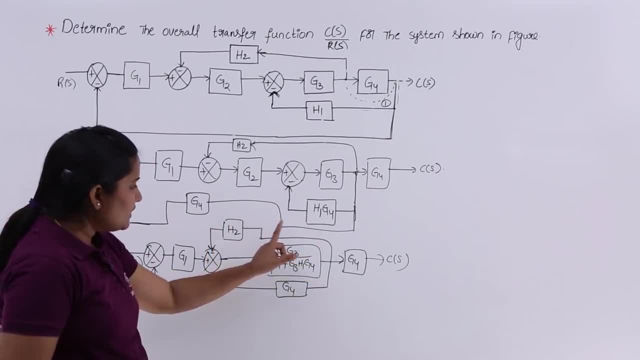 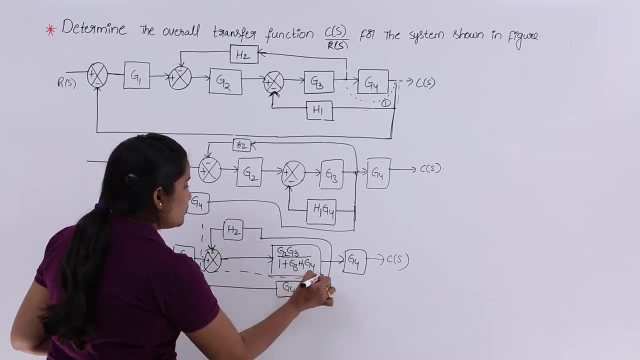 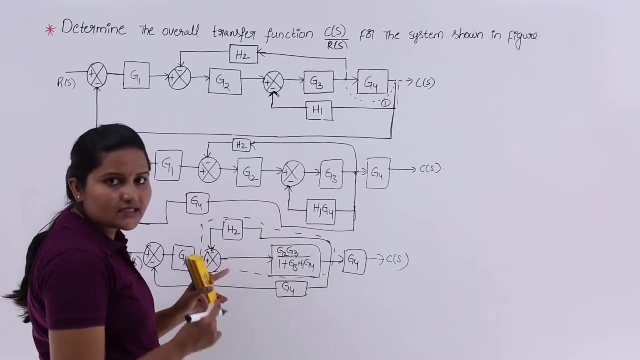 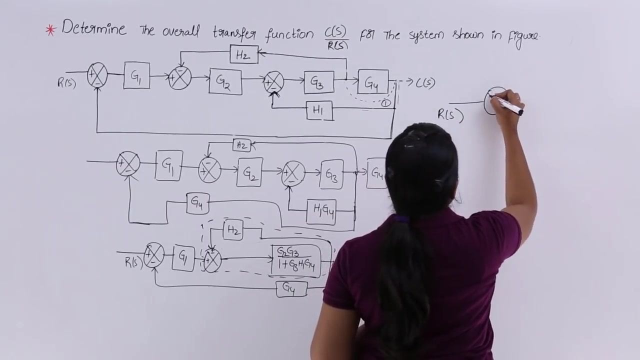 are having a feedback. That feedback is a negative feedback. So you can reduce this by using negative feedback gain. So that means you can make that total feedback path as feedback path gain. So now the reduced diagram is RFS. So you are having summing point plus minus and you are having G 1 here. 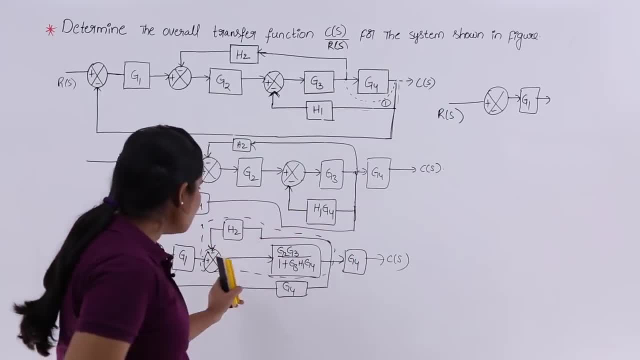 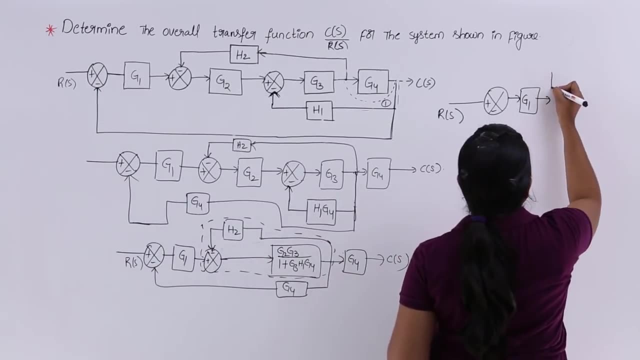 After G 1, you are having this feedback loop. So this feedback loop, that means with negative feedback, I can write this as G 3.. So G2, G3 divided by 1 plus G3, G4, H1 divided by 1 plus H2, into G2, G3 divided by 1 plus. 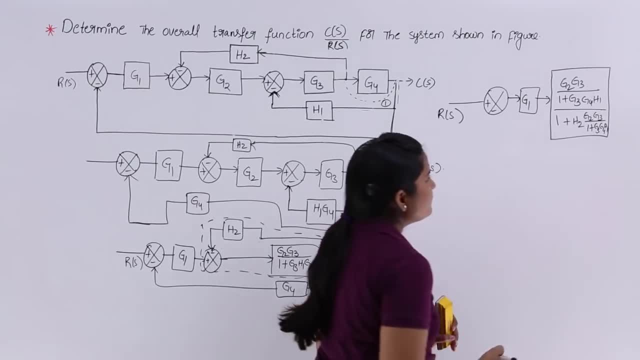 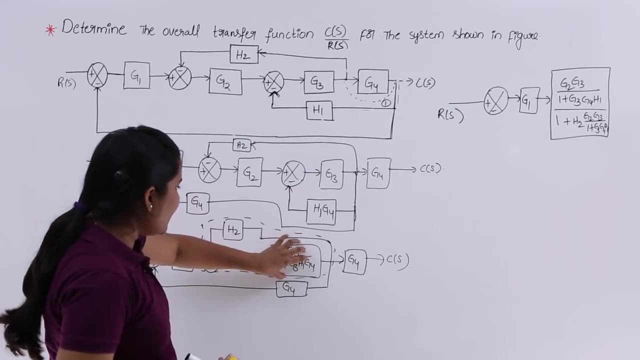 G3, G4, H1.. Now you can see. So, in place of this feedback, I written like this: G by 1 plus GH, This is open loop gain G. You just treat like this G, open loop gain, and this is feedback gain. 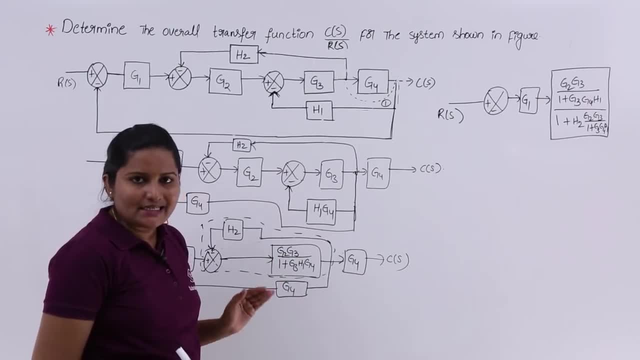 So negative feedback transfer function is equivalent to open loop gain divided by 1 plus open loop gain into feedback gain. So G by 1 plus GH, G divided by 1 plus G into H. So that form I written there. 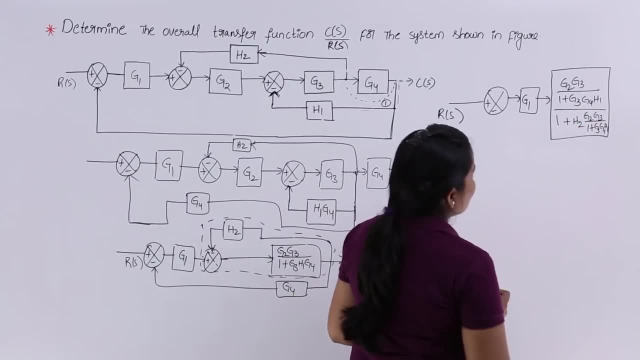 So now? So if you reduced this, what you are going to get? So I am just reducing this: G2, G3 divided by 1 plus G3, G4, H1.. So, divided by, I am cross multiplying this: 1 plus G3, G4, H1 plus G2, G3, H2 divided. 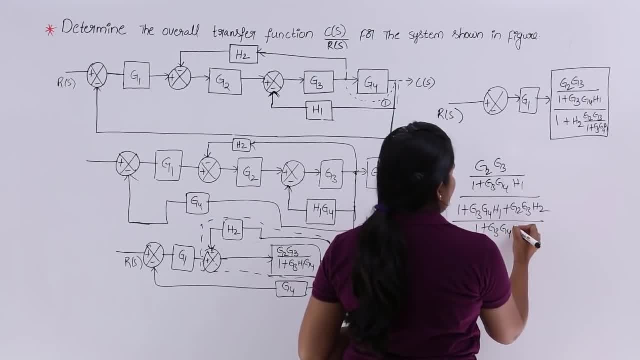 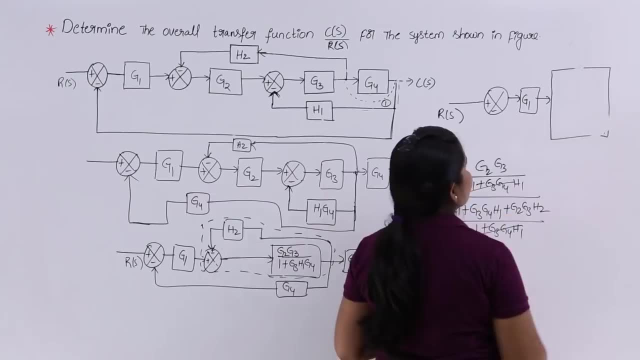 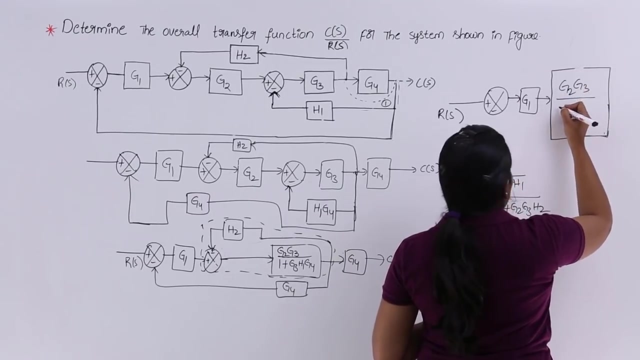 by 1 plus G3, G4, H1.. So these two I can cancel, the remaining I am writing here. So these two I can cancel, the remaining I am writing here. So the remaining is remaining is so G2, G3 divided by 1 plus G3, G4, H1, plus G2, G3, H2.. 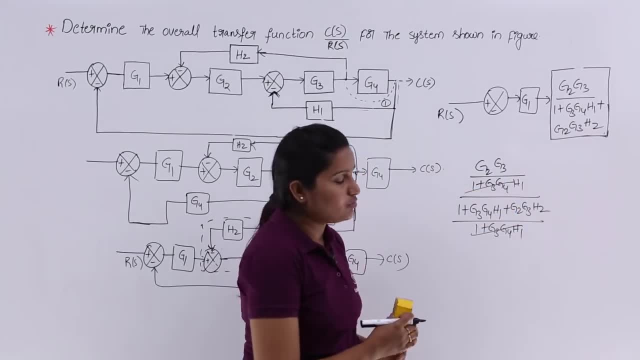 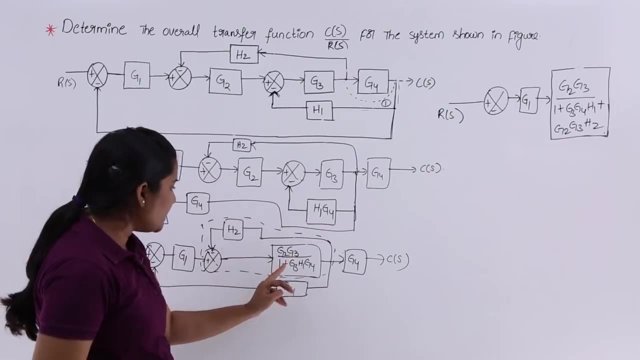 G3, G4, H1, plus G2, G3, H2.. So now, So I reduced this feedback path, I reduced this feedback path And I am having this G4 and then this feedback. So I am having this G4. 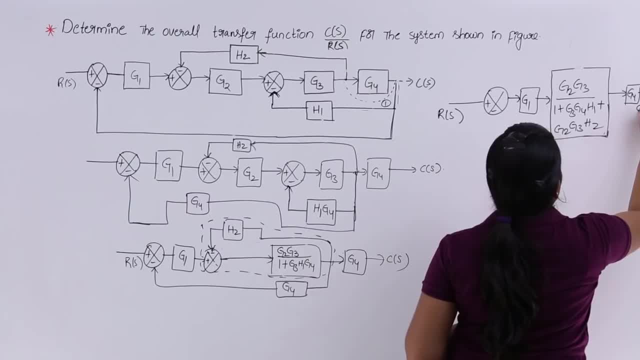 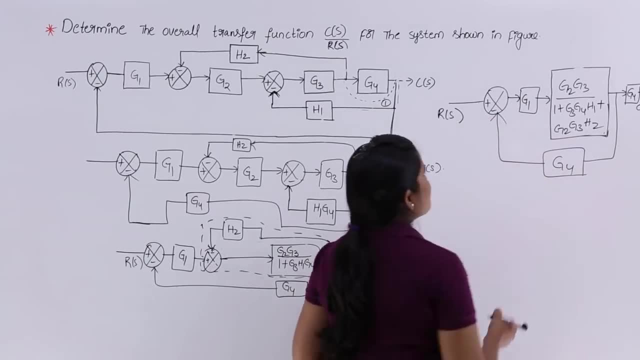 I am having this G4 and C of S, And here I am having feedback, another feedback, G4.. So, like this I am having. This is the my reduced block diagram up to now, So you can see these two blocks are in series. 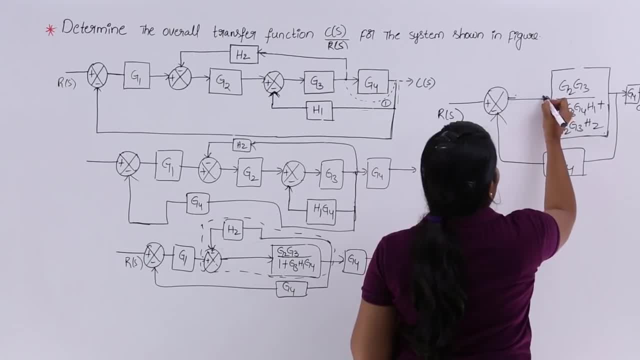 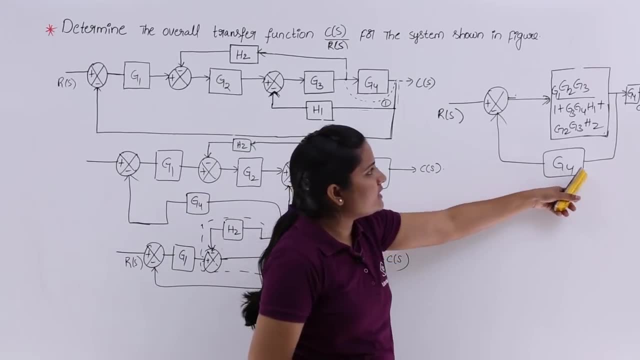 Definitely we can take out this block And we can make this a single block by multiplying G, G1, G2, G3.. And here this block is in feedback, So that is also negative feedback. Again, we can apply formula G by 1 plus GH. 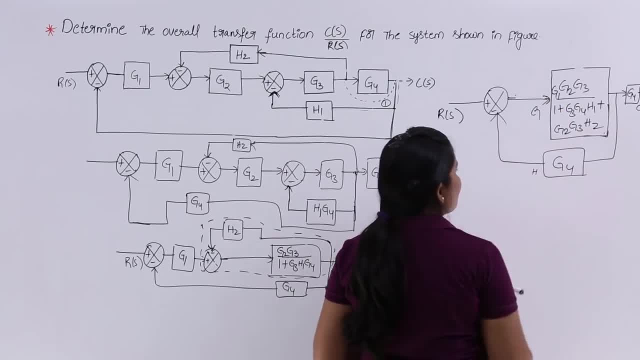 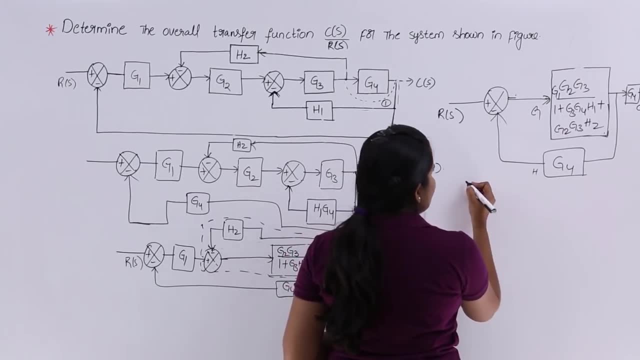 You just treat this as H and you just treat this as G, So I am writing that So that gain is equivalent to. first of all, I am solving that gain here. G by that means G1, G2, G3 divided by 1, plus G3, G4, H1. 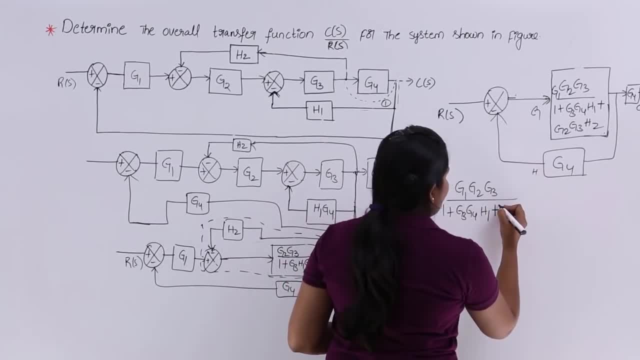 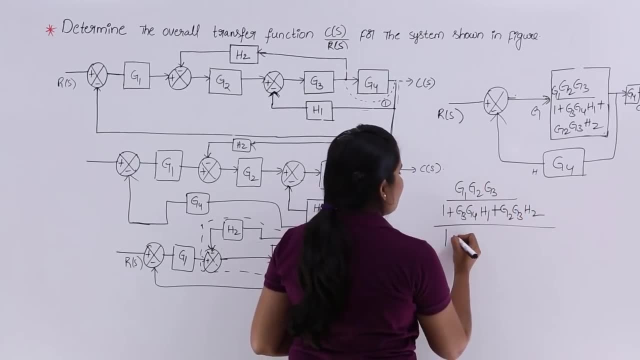 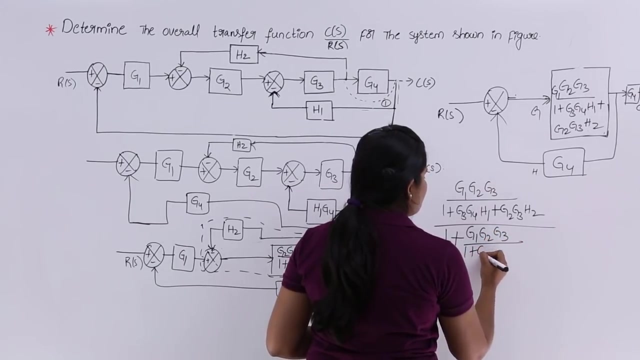 Plus G2, G3, H2 divided by, so G by 1 plus GH, So this G again, we need to write G1, G2, G3 divided by 1 plus G3, G4, H1 plus G2, G3, H2 into H, means in place of H I am having G4.. 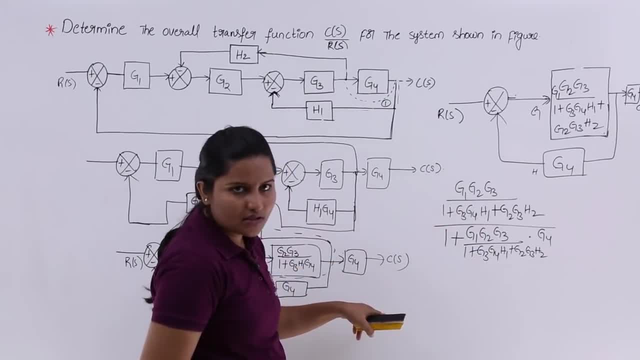 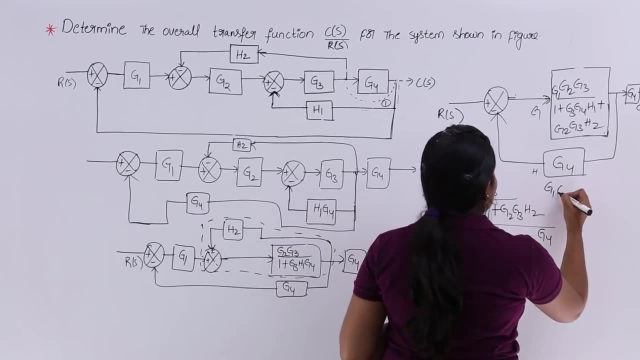 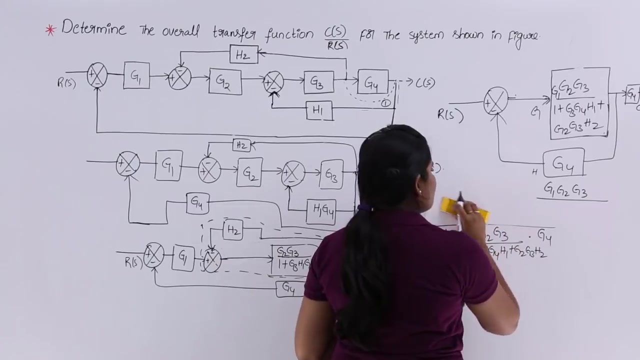 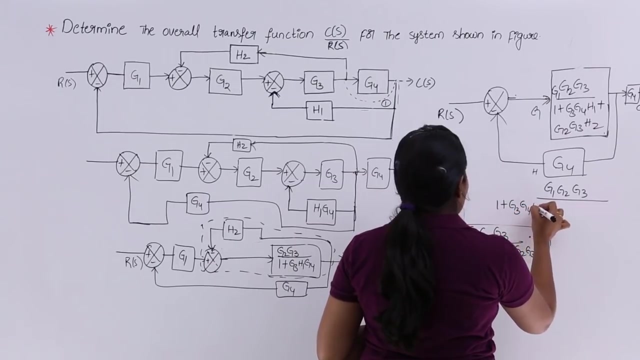 Just Cross multiply and cancel the denominators. Then you are going to get. so here you are going to get. so G1, G2, G3 divided by. So by cross multiplying you are going to get. you can see: 1 plus G3, G4, H1 plus G2, G3, H2 plus G1, G2.. 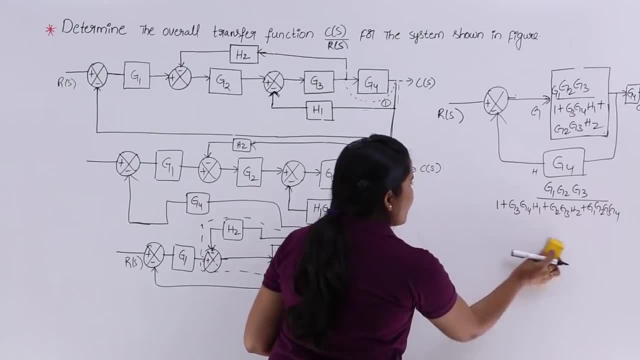 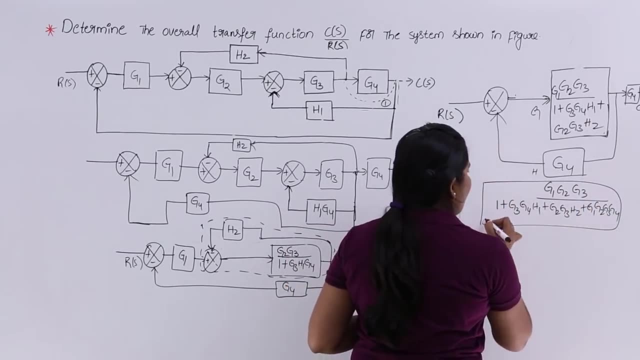 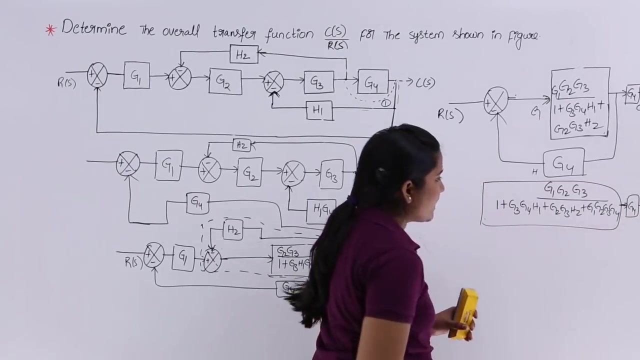 So this, what we are getting as gain by simplifying this feedback loop, we are going to get this as you are gain, and here you are having another G4, another G4 you are having. So this G4 you are having here, and here you are having R of S and here you are having C of S at the output of G4, and now by multiplying these two, you can see these two are series. 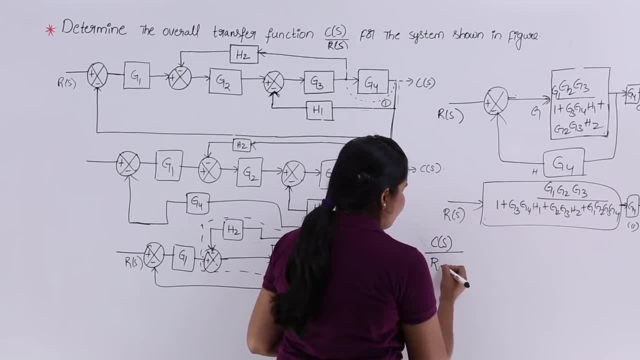 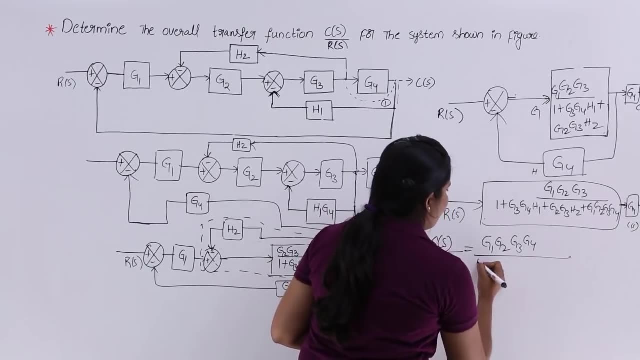 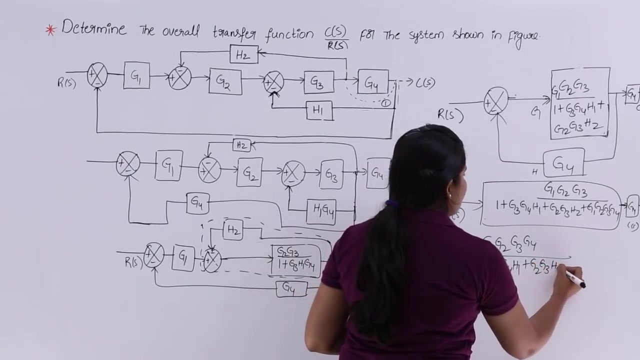 Block. by multiplying these two, you are going to get C of S by R of S. that means G1, G2, G3, G4 divided by 1 plus G3, G4, H1 plus G2, G3, H2 plus G1, G2, G3, G4.